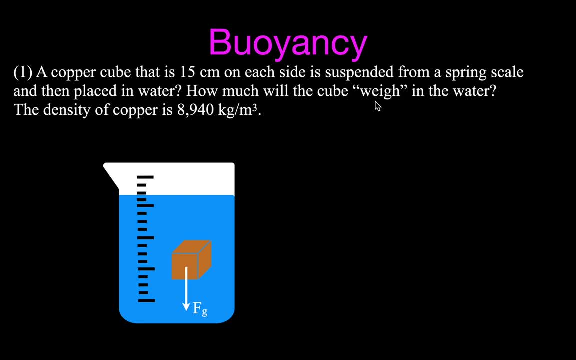 figure out what the buoyant force is going to be. because the weight is pulling down. You can see that Fg, that's the weight of the object, that copper cube- And we have the buoyant force because that pushes up in the opposite direction. So that means if we hang it from a spring, scale the force. 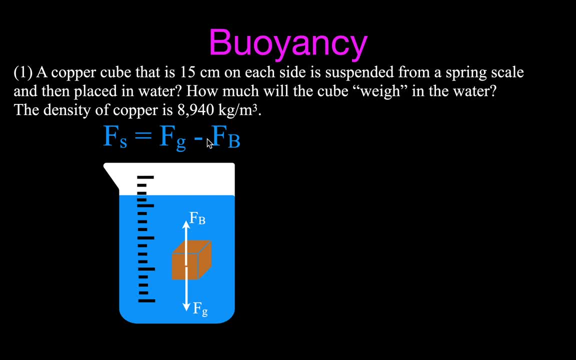 on the spring scale, Fs is going to be the weight minus the buoyant force. The weight pulls down and the buoyant force pushes up in the opposite direction. We can get the weight from Newton's second law: Fg equals, Fg equals Mg, And we can get the buoyant force from this equation, which 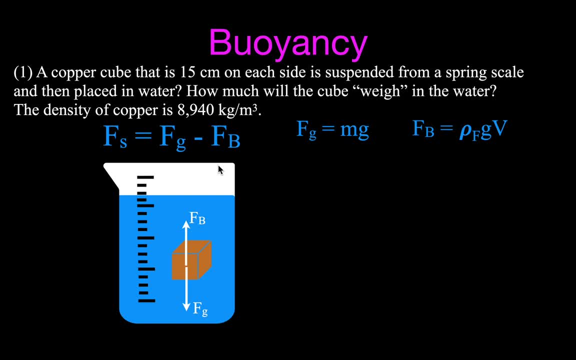 is that the density of the fluid, which is water in this case, is times the acceleration to gravity, which is the volume of the object or the volume of the water in this place, because they're the same, will give us the buoyant force. Now the weight of the object. we need to get the mass Now I gave. 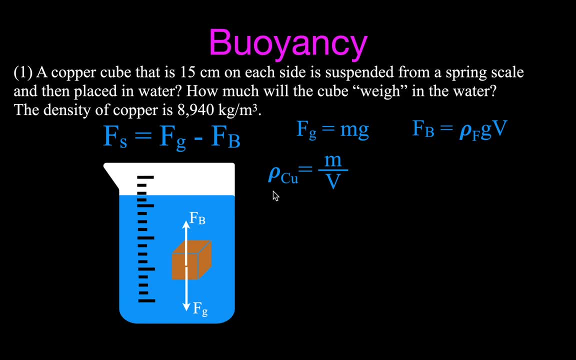 you the density and the volume. so you can get the mass from the density equation, which says that the density of copper is equal to the mass divided by the volume. We can rearrange that We get the mass is equal to the density times the volume. If we plug the values in, we get that the mass is. 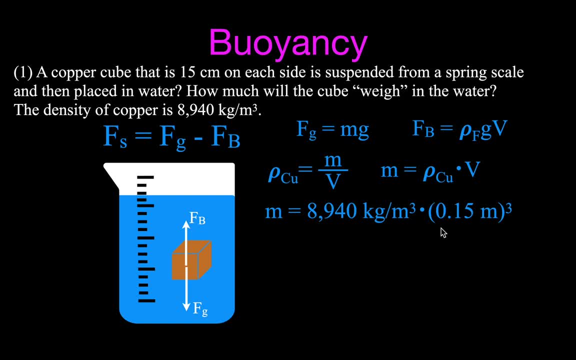 equal to the mass divided by the volume. If we plug this into meters- because this is centimeters, that's 0.15 meters. We cube that and we get that the mass of that cube is going to be 30.2 kilograms. 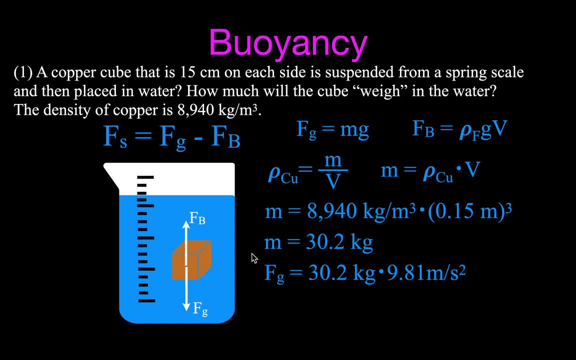 And now to get: the weight is 30.2 times 9.81 from this equation right here, And that gives us that that cube weighs 296 Newtons. So that is the weight. That's this value we need. Now we need: 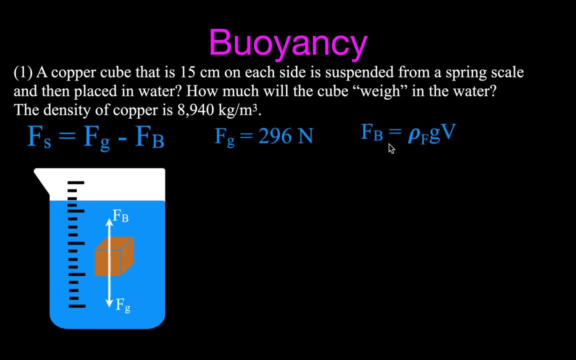 the buoyant force. We can calculate the buoyant force from our buoyant force equation which says: the density of the fluid, times g times the volume is equal to the buoyant force, which this is the density of water, 1000 kilograms per meter cube. This is acceleration due to gravity g and this 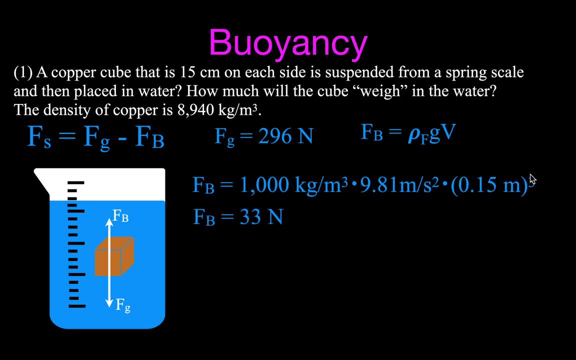 is the volume, once again in meters. We got to cube it and we get that the buoyant force is 33.. So now we have the weight, We have the buoyant force and the weight on the spring. The force on the spring scale is going to be the weight of the object which pulls down the buoyant force. 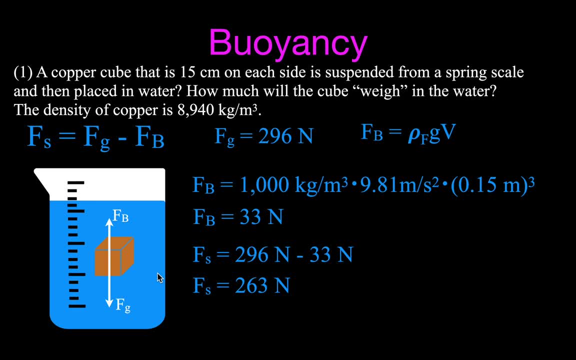 which pulls or pushes up, And we get that that cube in water. the apparent weight is 263 Newtons. That is the end of example number one, And now we can go on to example number two. And example number two has to do with the 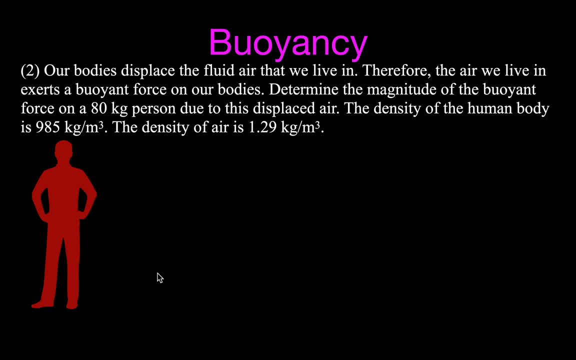 buoyant force on the body. Now, we don't often think about the buoyant force in air, but we are in air, which is a fluid, and it does exert a buoyant force. It's not very high, as you'll see. 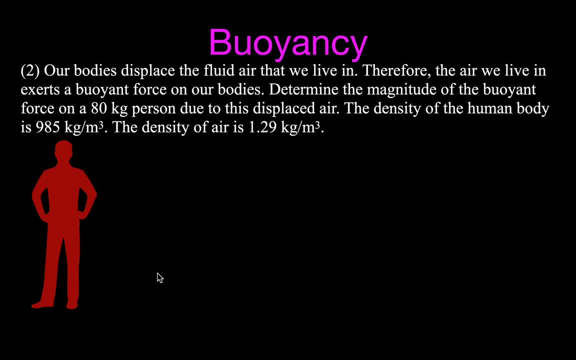 because density of air is not very high, But we can figure out the buoyant force on a person who has a mass of 80 kilograms. Here's the density of the human body, which I just looked this up. I found a few different answers, but I got these values And this is the density of air And we. 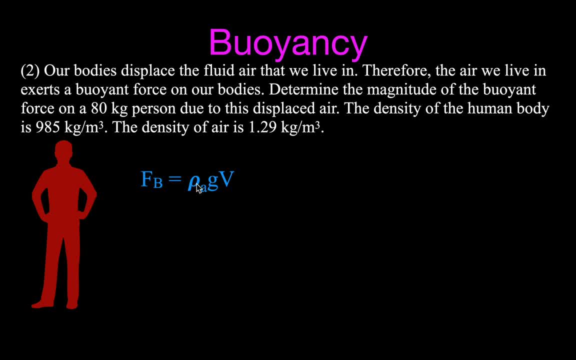 can get the buoyant force on that person is that the density of air. because you're in air times, g times the volume. Now, once again, I didn't give you the volume, I gave you the mass this time and the density, So you can get the volume of a person from the density equation. The density of a person. 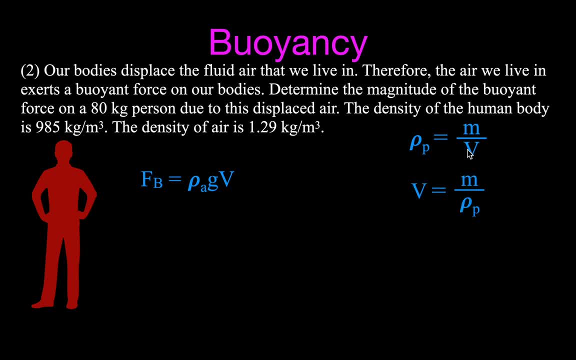 equals the mass divided by the volume. The volume would be the mass divided by the density, And that's 80 divided by 985 kilograms per meter cubed. You can see the kilograms cancel. You're left with 0.081 meters cubed. We can plug that into this equation, which is the density. 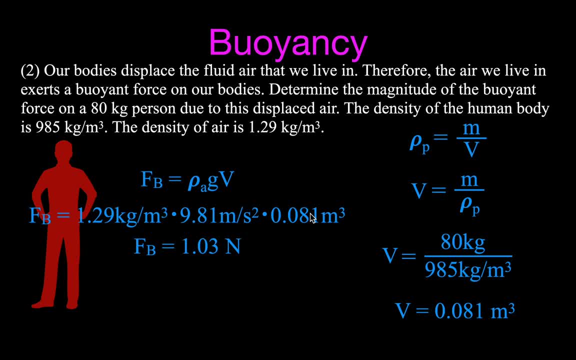 the acceleration and the volume And you get that the buoyant force. your weight really decreases by one Newton. when you're an 80 kilogram person approximately Now, is that a lot? I mean it's not a lot, but let's just see what that would be, maybe in pounds. 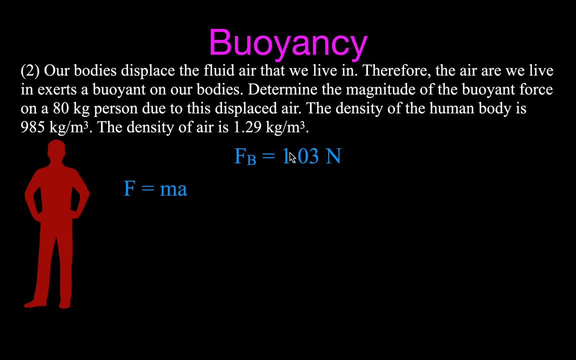 Okay, this is the buoyant force in Newtons And we can get the mass of that amount of weight in gravity due to gravity, by taking Newton's second law And we divide that We can take the mass is equal to the force This force is due to gravity. Therefore the acceleration is 9.81.. And we get: 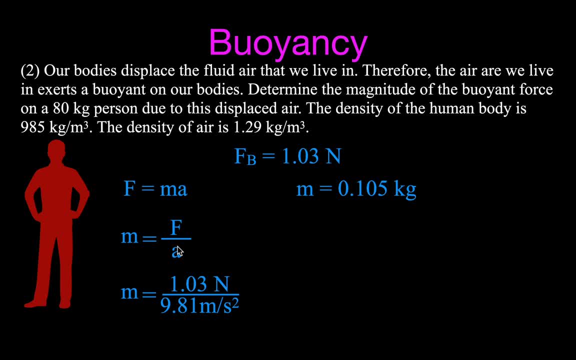 the mass is 0.105 kilograms, which is like 105 grams. How many pounds is that? Well, we can use this conversion factor, because one kilogram is about 2.2 pounds And we can see when you're in air you weigh a little less. You weigh 0.23 pounds less Now. 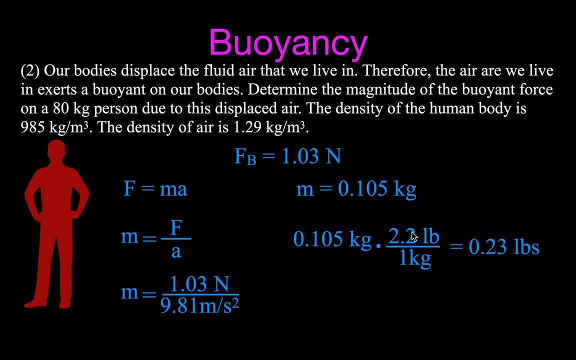 it's not very much. but if the air was to go away then you would weigh more and that wouldn't be good. But if the air was to go away then you would also be dead, so it wouldn't really matter. 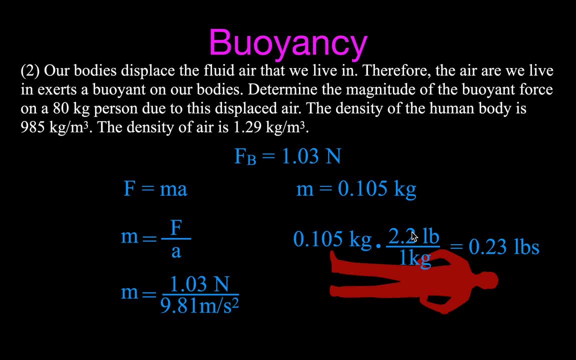 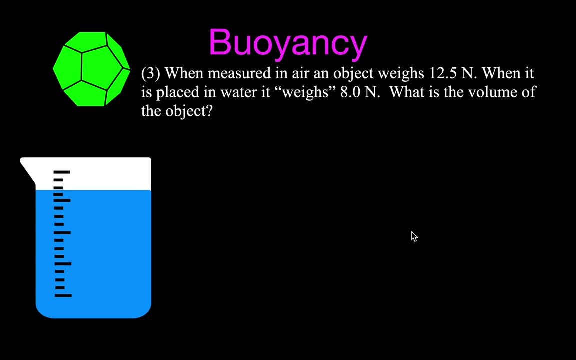 Okay, so there you go. That's example number two. Now example number three is: we have this object and when we measure it in air, when we weigh it, it weighs 12.5 Newtons. Okay, so that's. 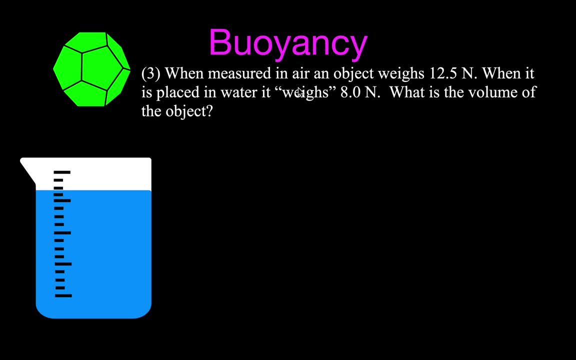 8 Newtons, Then we're going to place it in water and its weight, its apparent weight, is 8 Newtons. We want to know what is the volume of the object. Okay, everything has a weight on Earth When we 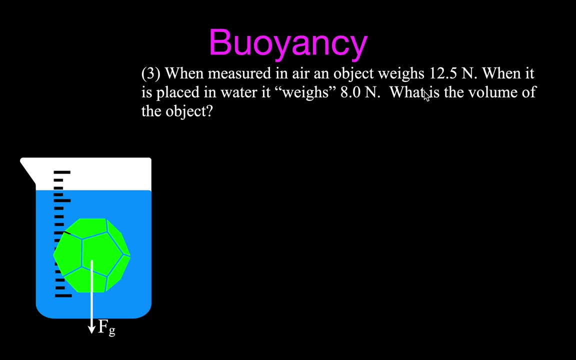 put it into water, it still has that weight, but we say it doesn't weigh the same because there's the buoyant force which pushes it up in the opposite direction. Okay Now the buoyant force is the force in air minus the force in water, And therefore the buoyant force is 4.5 Newtons. We can. 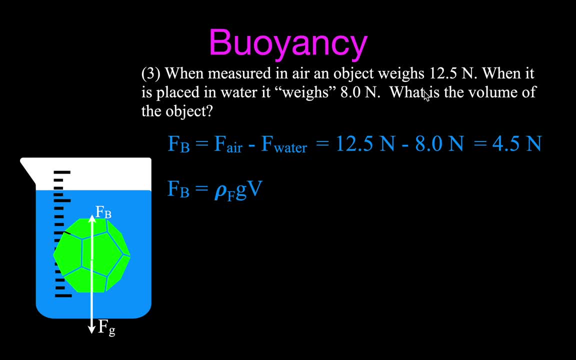 subtract those two, We don't need to use the other buoyant force equation. We want to know the volume. So here's the buoyant force equation and there's the volume that we're going to solve for the volume. And when we solve for the volume we get. the volume is the buoyant force divided by the. 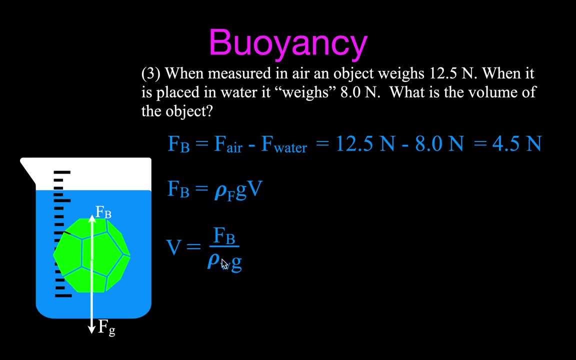 density of the liquid that it's in the fluid that it's in, which is water. So that's the density of water times g, And therefore we get that 4.5 Newtons divided by 1,000 times 9.81.. So the volume 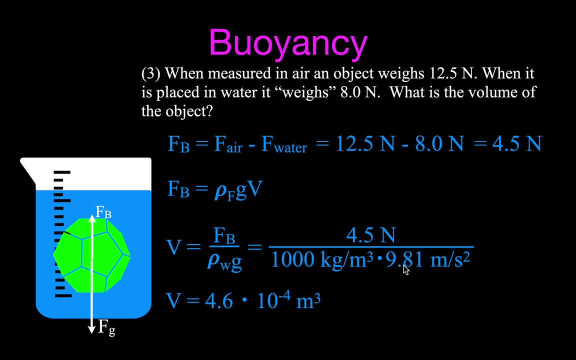 of that object is 4.6 times 10 to the minus 4 meters Supers cube. that kind of corresponds to that buoyant force like that when we have those two weights in air and in water. Okay, That is example number three, And now we can go on to example. 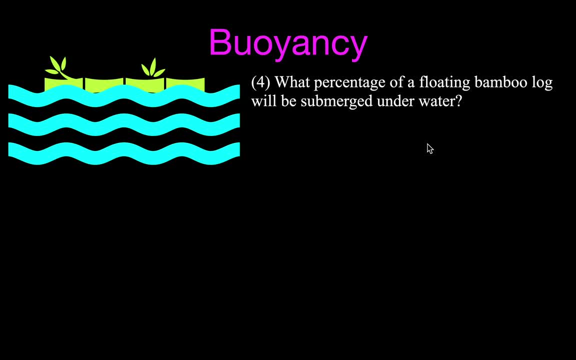 number four, which is a floating object. So this object is not submerged in water. It's floating and we want to know. it's a piece of bamboo, We want to know what percentage of it is actually submerged in water. Okay, density of bamboo is 620, the density of water is 1,000.. Now, you might know this intuitively. 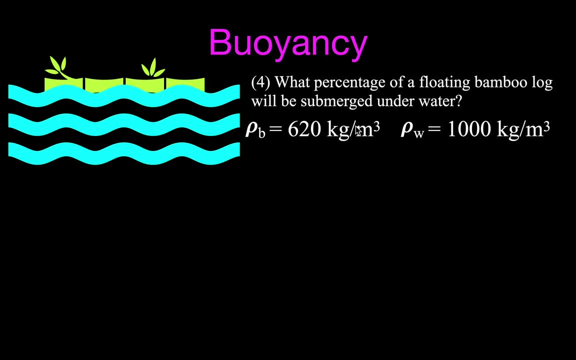 or you might see that maybe it makes sense that the answer is probably going to be 620 and 1,000. That's right. It's going to be 62%, right? If you had something that has a density of half of water, then half of it will be in the water, half of it will be above the water. 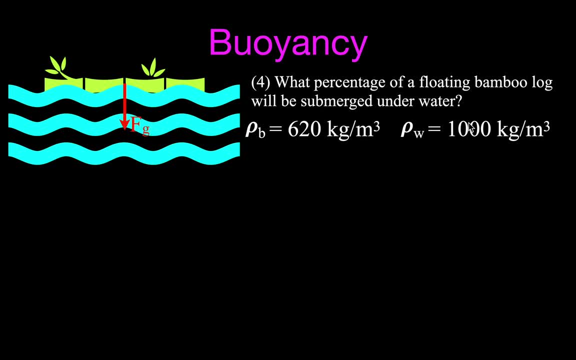 But we can actually use the Boeing force to come up with the answer to that and see where we get that 62%, because we know that the bamboo has a force of gravity acting on it and if that object is floating then we know the Boeing force is equal. Those two forces are equal to each other. 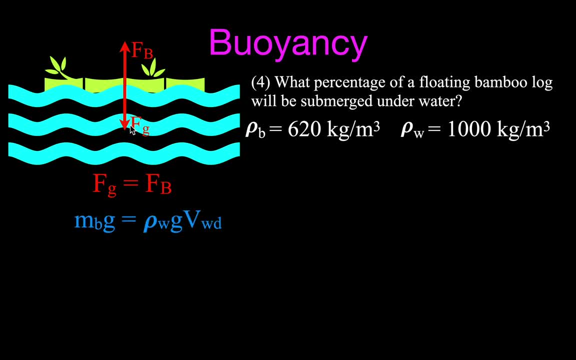 the force of gravity and the Boeing force. And the force of gravity is the mass of the bamboo times g, which is equal to the Boeing force, which is the density of water, because it's in water. times g times the volume of the water that is displaced When something is floating. 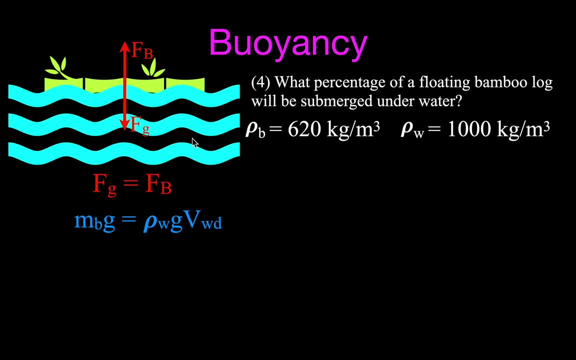 we use the volume as the volume of the water That's displaced. It's always the volume, but in this case it's not completely submerged. Okay, so now we can put in here. you can see. here's the mass of the bamboo. 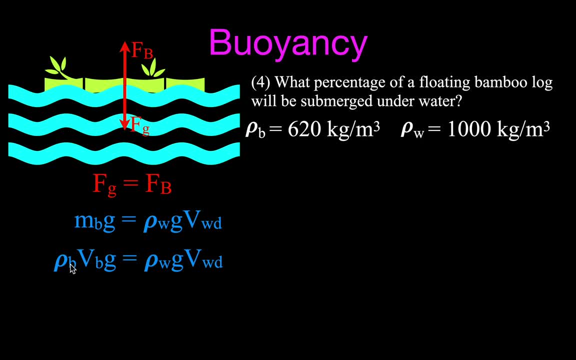 Okay, we don't know the mass, Okay, but here you can see we can substitute in the density of the bamboo from again from the density equation, that the mass is the density times the volume, And you can see that we have g on both sides, So we can factor that in. 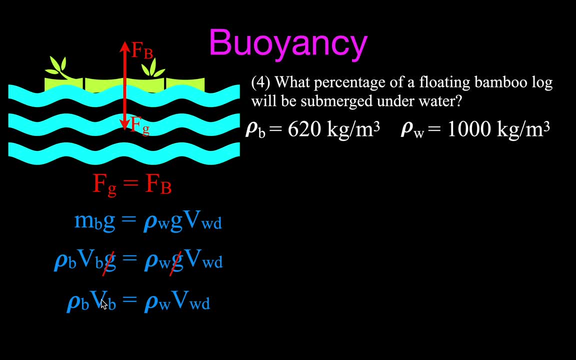 We can cancel g. That means we're left with the equation like this: The density of bamboo, volume of bamboo is going to be equal to the density of water times the volume that is submerged, which is the same thing. Those two volumes are going to be the same And we can. 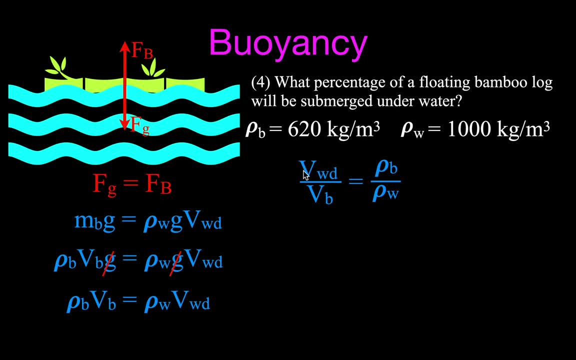 not the same, but we can take the ratio of the two. The ratio of the volume of that is submerged, displaced there, divided by the volume of the bamboo, is equal to the density of the bamboo divided by the density of the water. And therefore we can take that ratio and we can. 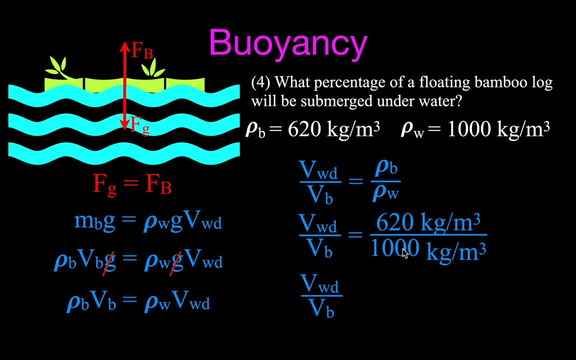 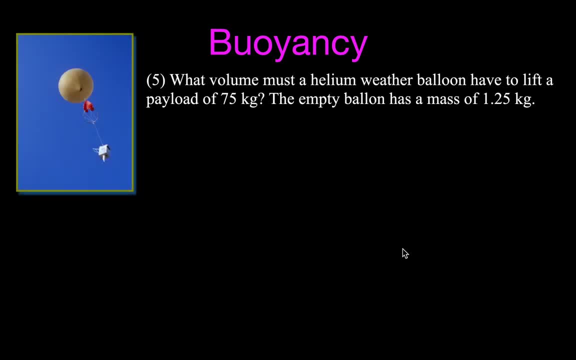 divide the 620 by the thousand and you get 62 percent or 0.62 or 62 percent. So that means the bamboo would 62 percent of it would be underwater. Okay, now we have the last problem And the last. 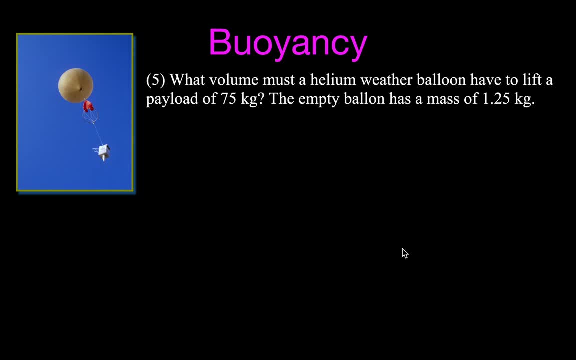 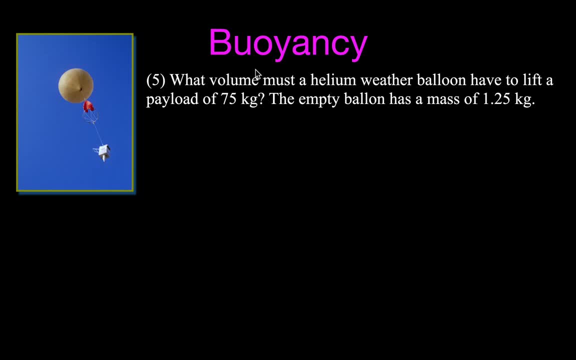 Okay, I put here weather balloon And it wants to lift the payload of 75 kilograms. Okay, and the balloon: we're going to take into account the fact that it has a helium balloon And the balloon actually has some mass. So the mass of the balloon is 1.25 kilograms. This is the density of air. This. 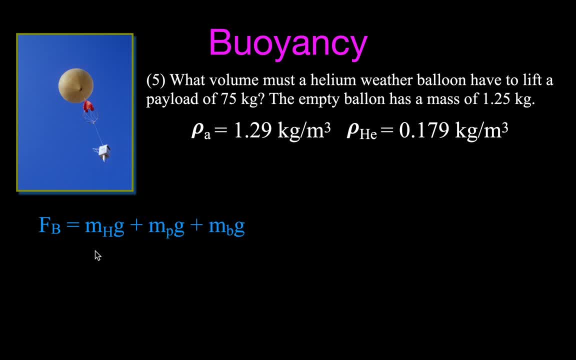 is the density of helium, And we know that the buoyant force. buoyant force has to lift those things up, So it has to be more than the weight of the helium. Now, I didn't put He here. This is not hydrogen, This is helium: H for helium. 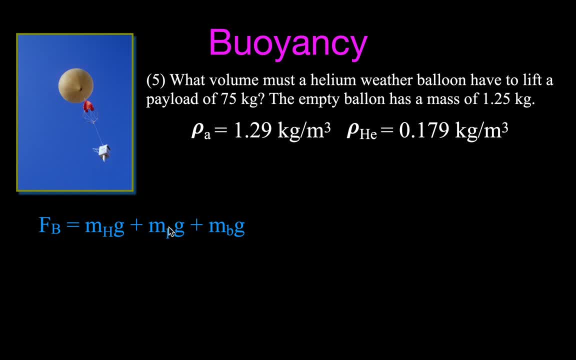 Then this is the mass of the payload, or the weight of the payload, And this is the weight of the actual balloon. Now we know the buoyant force is the density of the air times, the volume times, g. Okay, We have a g in all of these terms. We can factor that, cancel that g out And now we're left. 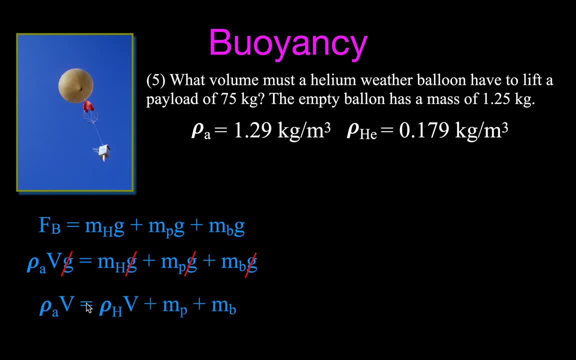 with this equation, which is the density of air times, the volume is equal to, okay, density of the helium: times the volume, times the volume, okay, So this is the mass of the air times, the volume, And times its volume and the mass of the payload. 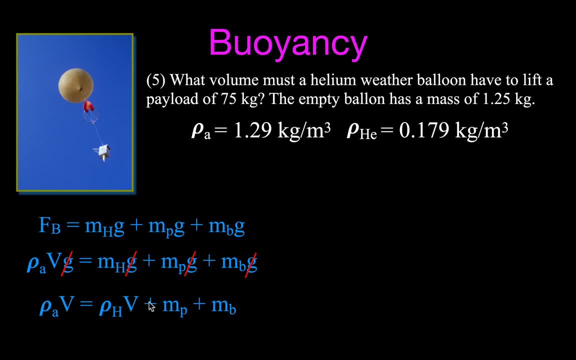 and the mass of the balloon. Now I'm going to do two things. We want to solve for the volume. We have two volumes here. They're the same volume, So I am going to subtract this term from both sides to get it to the other side. 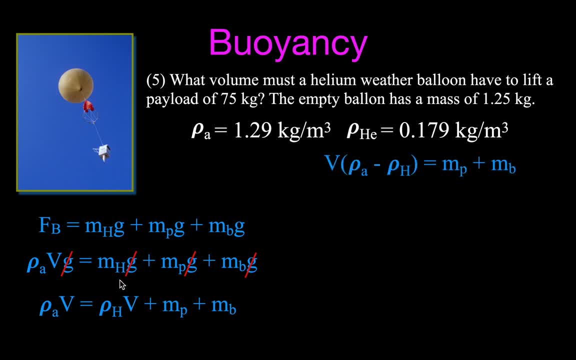 and I'm going to factor the volume out And therefore I get that the volume times the density of air minus the density of helium- because I subtracted this from both sides, so this makes this a negative term- is going to be equal to the mass of the package. 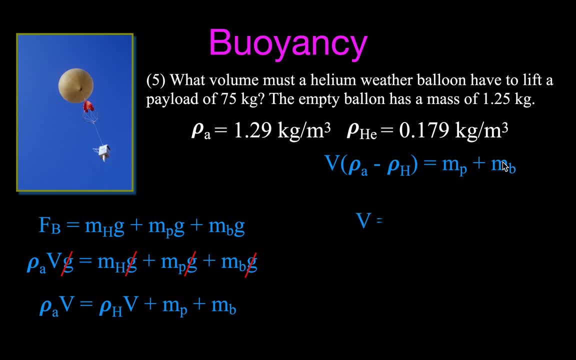 times the mass of the balloon- not times, but plus the mass of the balloon. And then I'm going to solve for the volume, which means I'm going to divide both sides by this term, the density terms here- And I get that the volume of the balloon. 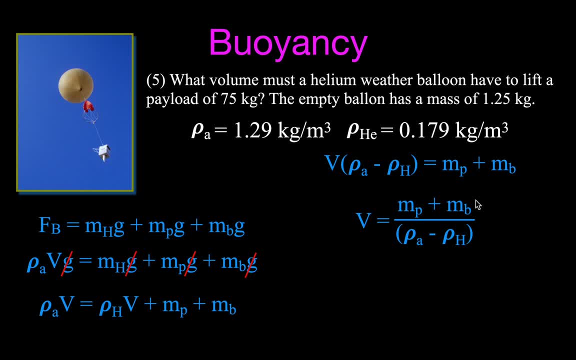 is equal to the mass of the package plus the mass of the balloon, which we're both given, divided by the density of the air minus the density of the helium, This is helium again. All right, and those are given too, So we know if we plug those values in. 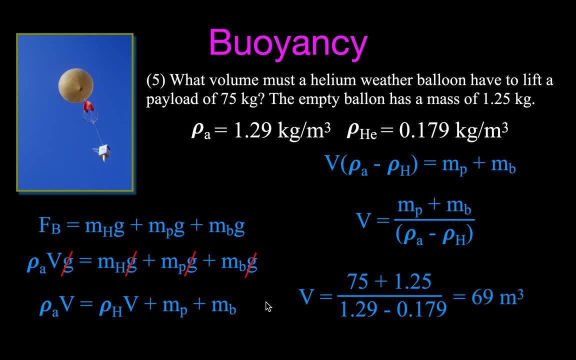 that we end up with just about 69 meters cubed. So in order, at the surface of the Earth, for a balloon to lift up itself and the package and the helium that's in the balloon, because you've got to take that into account. 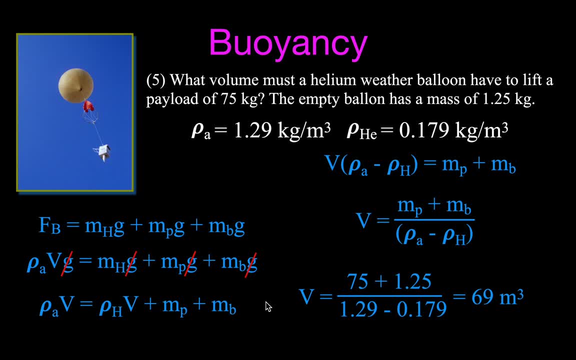 here we did. you're going to need a balloon that has a volume of about 69 cubic meters. Okay, So there you go. We did five exercises, Excellent examples covering a range of possibilities for buoyancy and Archimedes' principle. 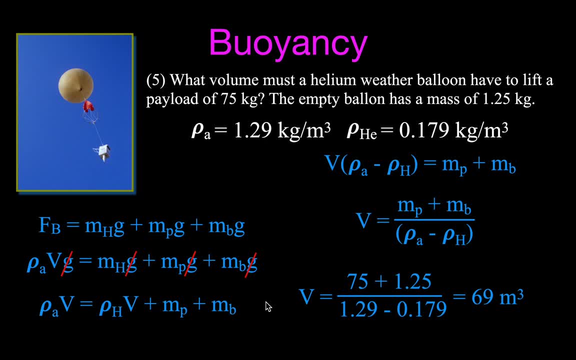 I hope that you found that video helpful. If you did, please don't forget to do all of the following five things: Support our channel, Step-by-Step Science. Please subscribe. Click the notifications bell so you don't miss anything. Leave us a nice, positive comment. 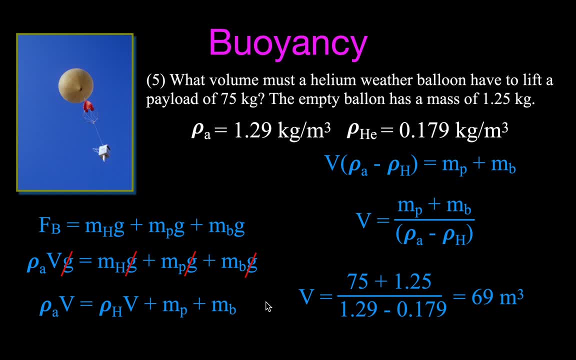 a thumbs up and don't forget to share this video. Thank you so much for watching. We will see you in the next Video. 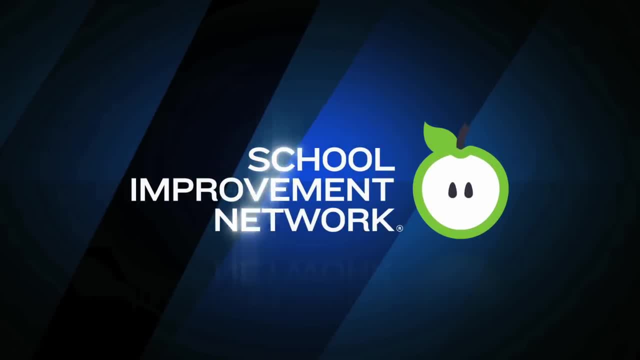 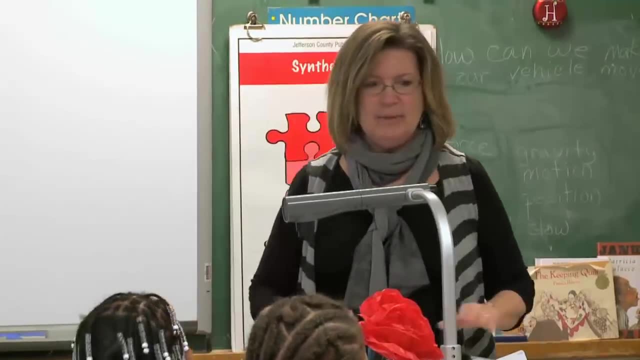 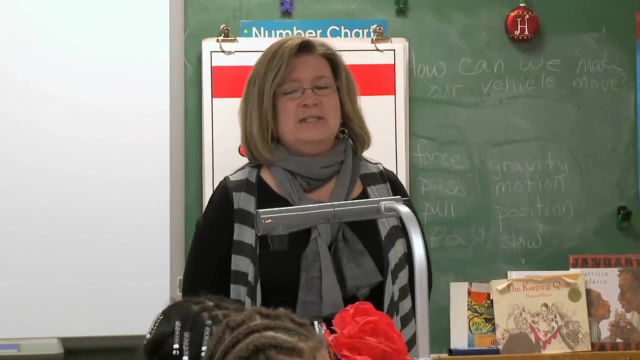 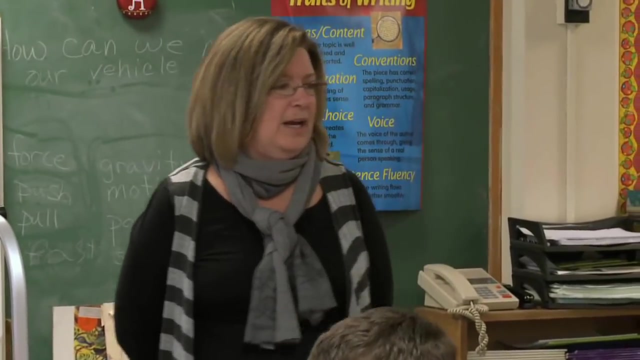 Okay, guys, we're going to get back into science. I know we've done some reading. Where is your science journal, All science journals? I'm seeing about three people without their journals on their desks. Okay, good, good, And I see those prepared, Excellent, Okay, who can tell me? 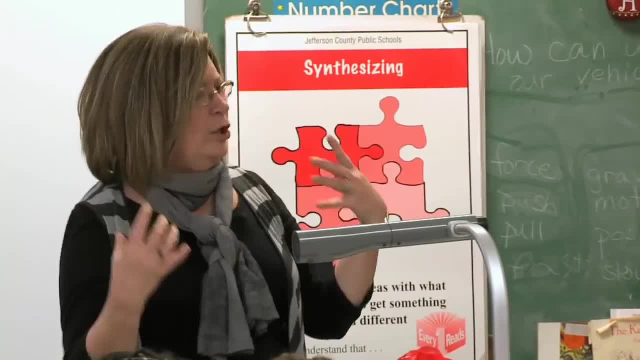 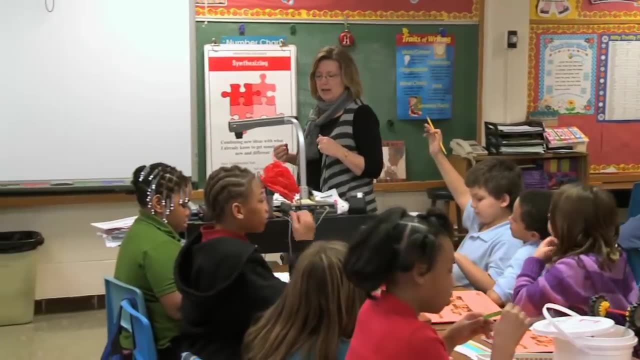 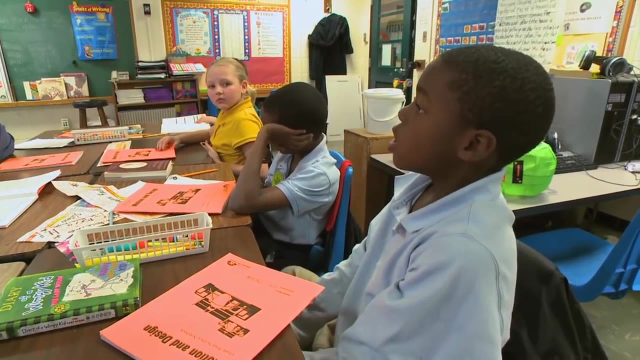 what we have been, what unit of study we've started in science. Who can tell me? Yes, Motion and design, Motion and design. What is motion? What does that mean? Yes, It has like forces. It's forced. What do you mean? motion has force. What do you explain what you're?